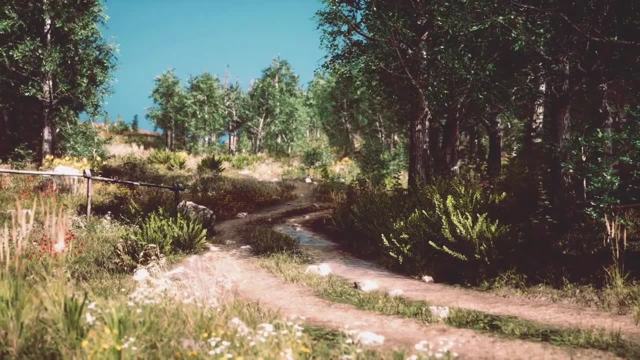 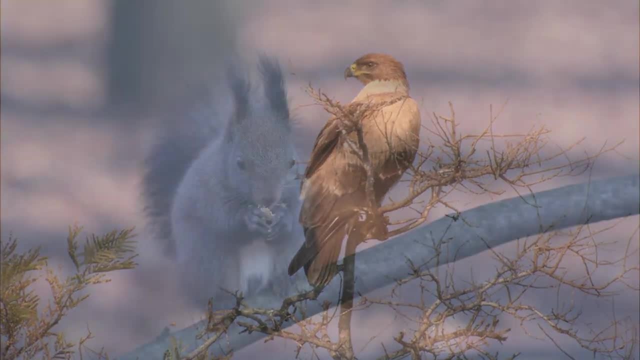 some trees, grass, dirt, a few rocks, sunlight or even rain clouds. There may be some birds in the trees, or squirrels. Can you identify the biotic or living factors? Remember that in order to be alive, organisms can be living or not living. So if you live in a temperate climate, 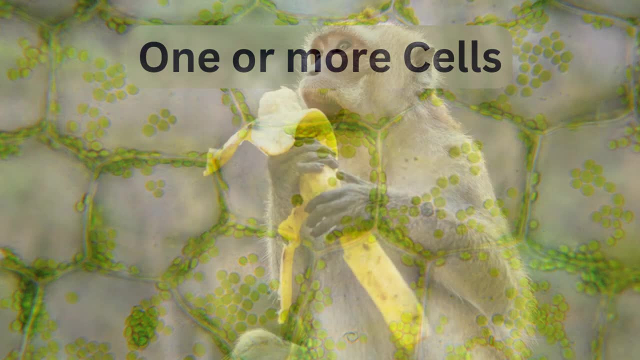 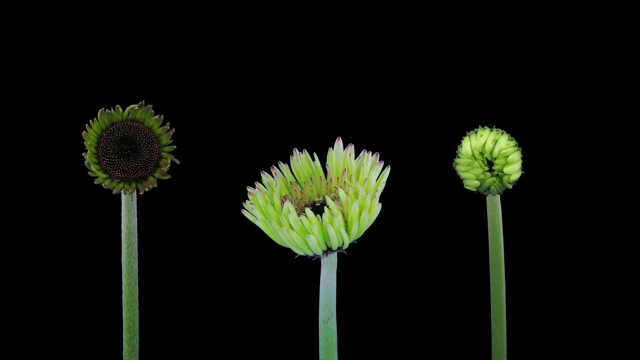 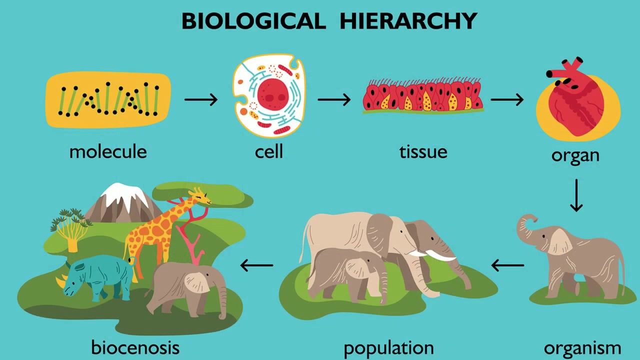 organisms must have cells, consume energy, be able to regulate their systems or maintain homeostasis, have the ability to grow. they must have the ability to sense their environment and respond to stimuli, and have levels of organization and be able to reproduce. 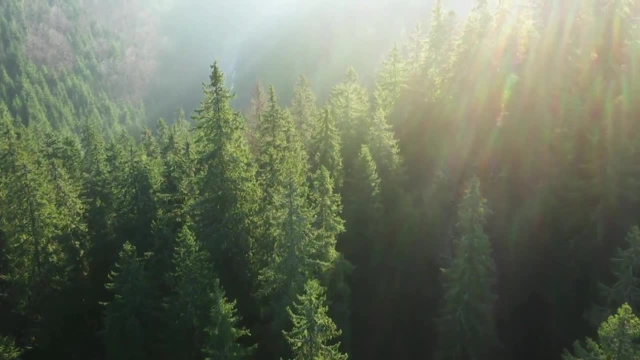 So how about trees? Are they alive? A tree starts as a tiny seed and grows into a towering giant. Tree cells are alive. A tree starts as a tiny seed and grows into a towering giant. Tree. cells are alive. Tree cells are alive. A tree starts as a tiny seed and grows into a towering giant Tree cells form. 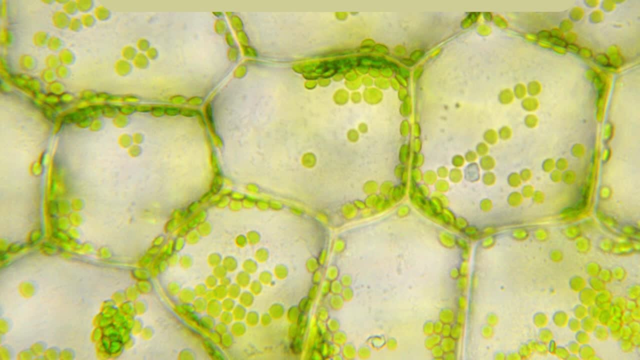 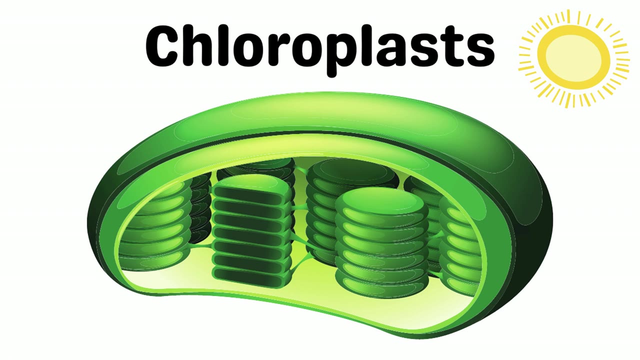 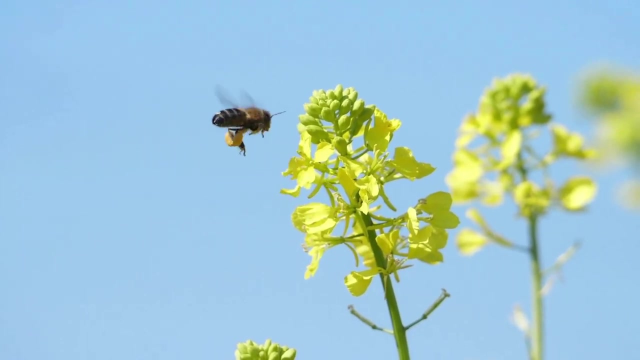 together to give them specific structures or levels of organization. Trees have specific cells called chloroplasts that allow them to take in sunlight and convert it into energy using photosynthesis. Trees are capable of reproducing through pollination and spread their seeds. They maintain homeostasis by regulating the amount of water held in their 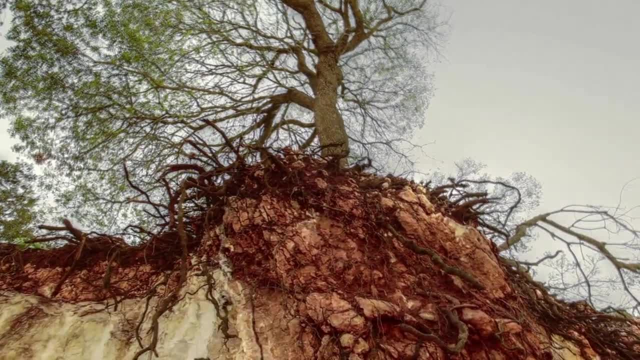 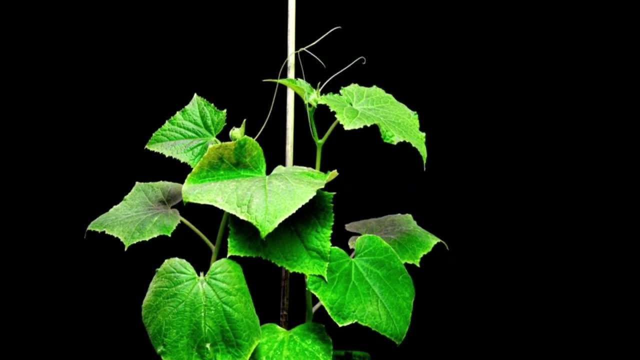 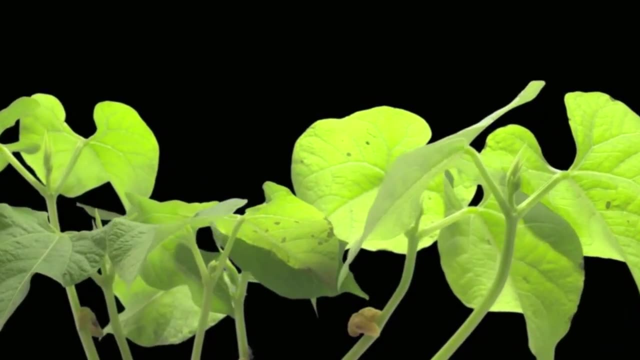 branches and leaves. They allow water to evaporate from their leaves to keep themselves cool. And lastly, trees are capable of responding to their environment. Most plants, including trees, exhibit phototrophism, meaning they turn themselves and grow in the direction of sunlight. So trees also demonstrate. 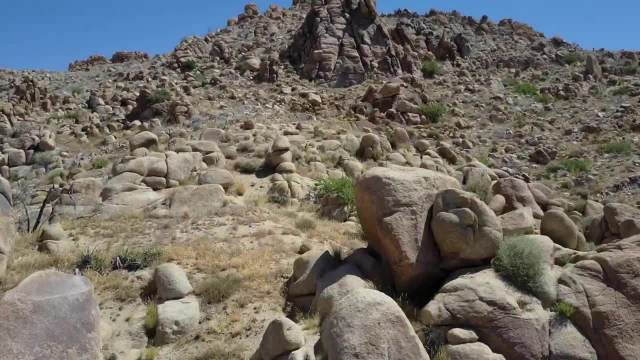 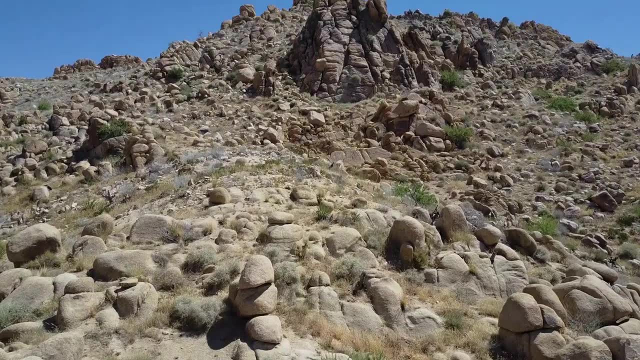 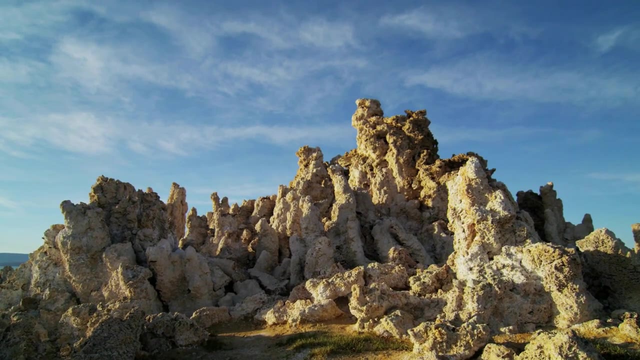 all the characteristics of living things. How about rocks? Can a rock reproduce? No, you can break a rock into smaller pieces, but it cannot reproduce on its own. So you can stop there once you have determined that an object does not possess any one of the seven characteristics. 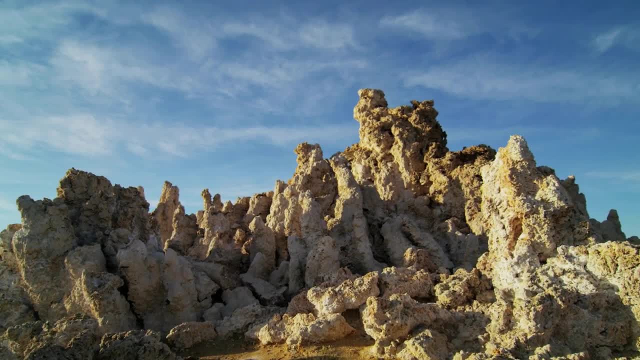 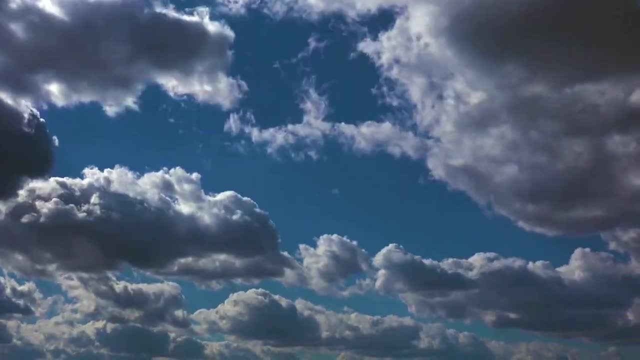 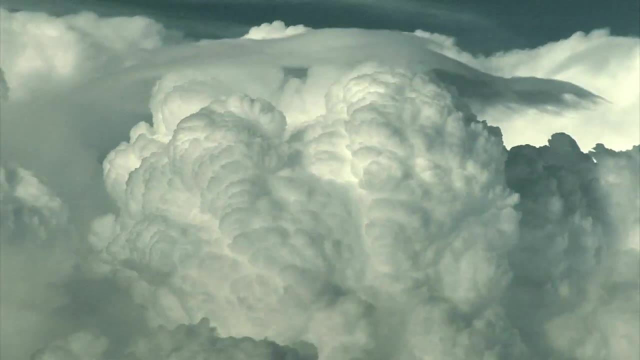 of living things – a non-living or an abiotic factor. How about clouds? It would seem like clouds may be living — they move, change sizes, have a general structure. However, clouds are non-living or an abiotic factor. They need the wind to push them. They are not capable.